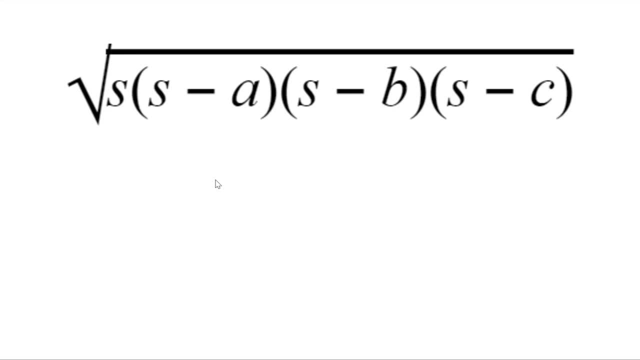 of thing that you learn about in school but you never really get a satisfying proof. that really explains why. There are a number of proofs to Huron's formula that you could have learned, but they're all trash because they're a disgusting bash and you know it's true because it rhymes. 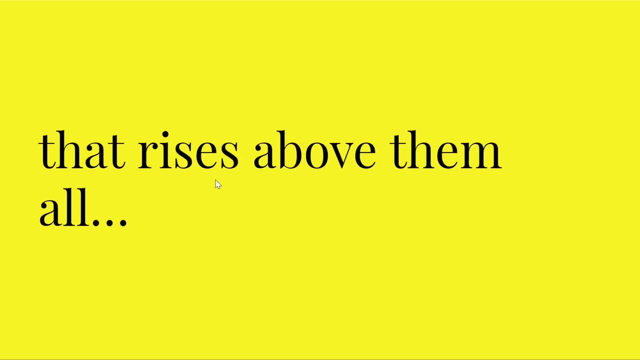 However, there is one proof that rises above them all. For some reason, most people don't know this proof, but it's much more elegant than the algebraic or trigonometric ways and doesn't include trig, And if you do know this proof, well then watch this anyways, because I need watch. 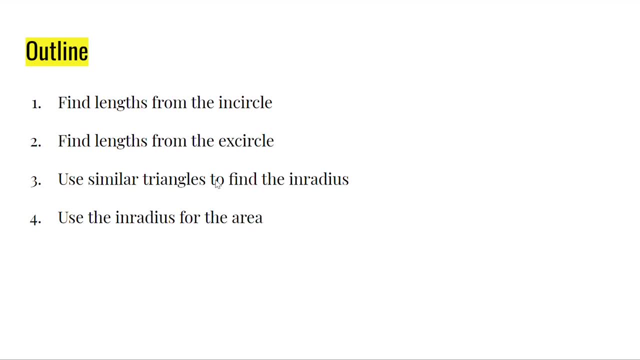 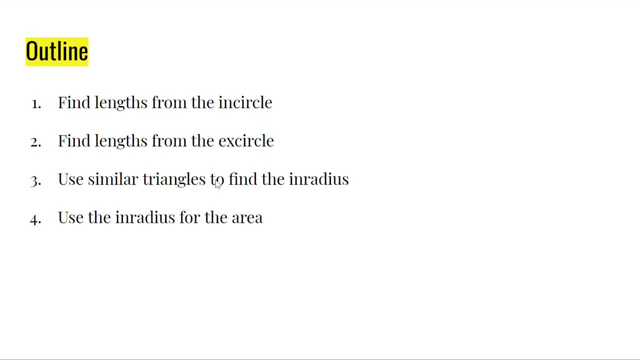 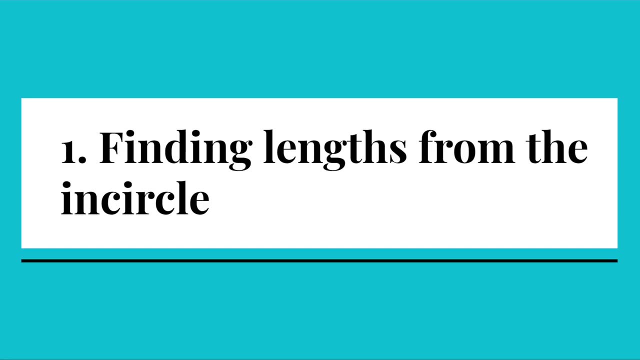 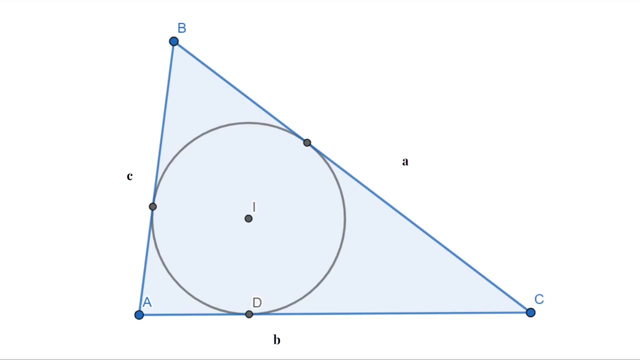 Now we'll find lengths from the in-circle. Next we'll use similar triangles to find the in-radius and finally we'll use the in-radius for the area Part 1, finding lengths from the in-circle. Let's start with a triangle ABC with side lengths A, B and C Inside of that. 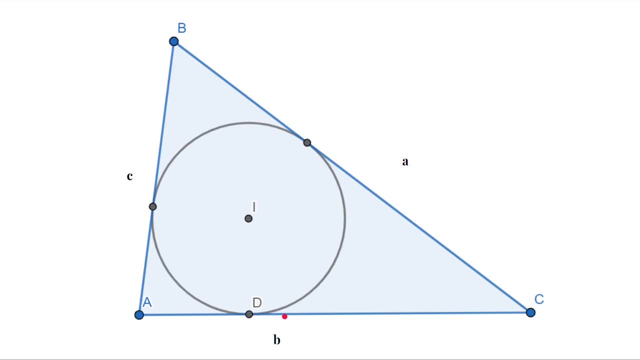 we'll put the in-circle, which is the circle that fits snugly inside and hits each of the sides, in exactly one point. Let's find the lengths from those points to A, B and C. This may seem like an impossible task, but we can use this key fact that the red segments are equal the green segments. 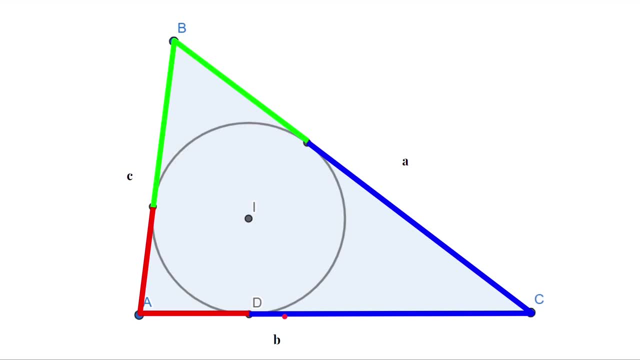 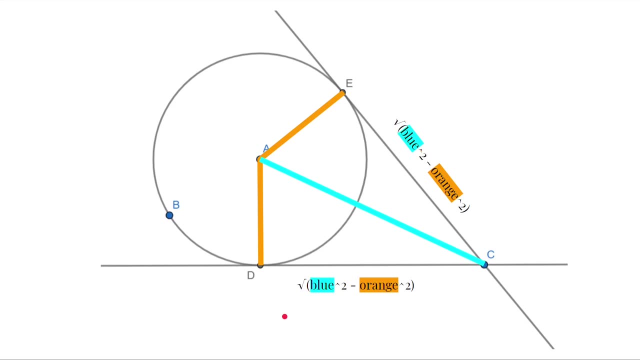 are equal and the blue segments are equal. This is because of a very special theorem. And what is this theorem called The Ice Cream Cone Theorem? Bet you won't forget it now. Actually, though, I don't think anyone calls it that except me. 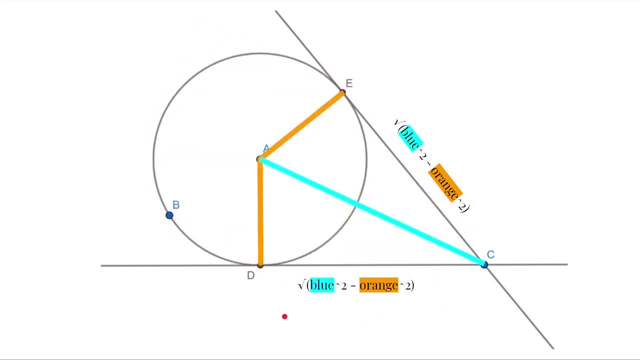 See, Looks like an ice cream cone. You can prove it easily by seeing that both of these angles are 90 degrees and the orange and blue sides are the same. So the Pythagorean Theorem says that the tangent lines CD and CE both have lengths square, root of blue squared minus orange squared. 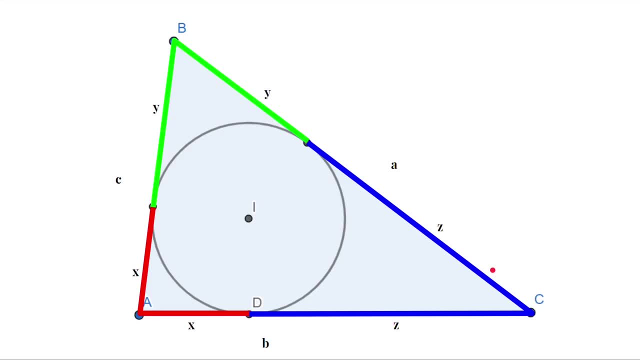 So they're equal. Let's call these lengths X, Y and Z. We want to find X, Y and Z in terms of A, B and C. Looking at each of the sides, we know that Y plus Z equals A, X plus Z. 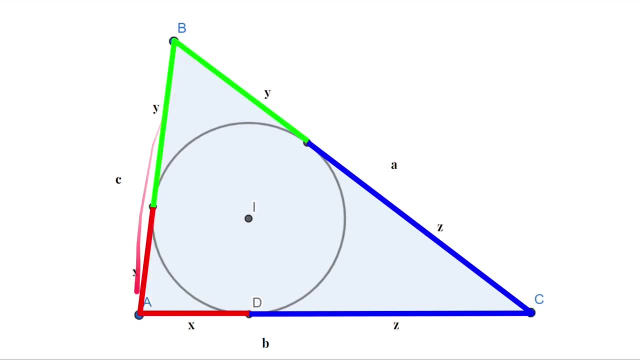 equals B, And X plus Y equals C. So now we have three equations and three unknowns. There's a lot of ways of solving for X, Y and Z, but the easiest is to first add the three equations and then 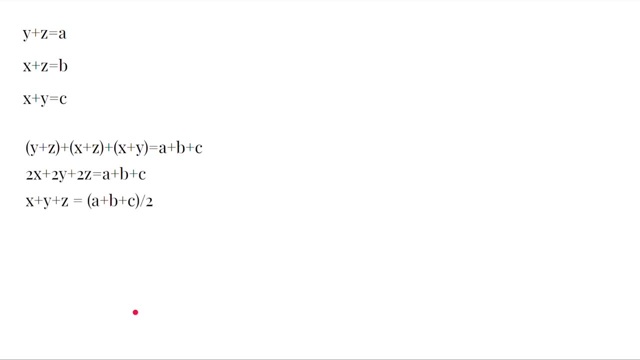 divide by two to get X plus Y plus Z. Like we can let X be equal to A plus B plus C over two, called the semi-perimeter or half the perimeter, because we'll end up using it a lot. So, subtracting each of the original equations from this one, we get: 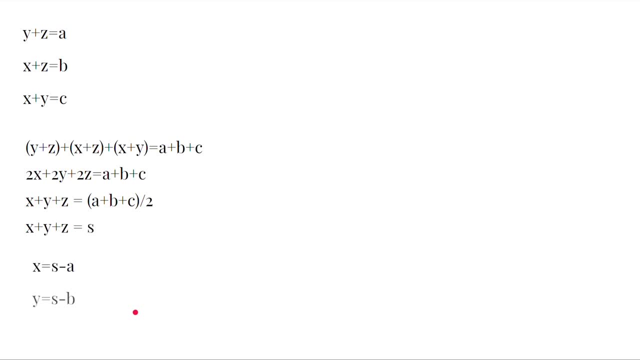 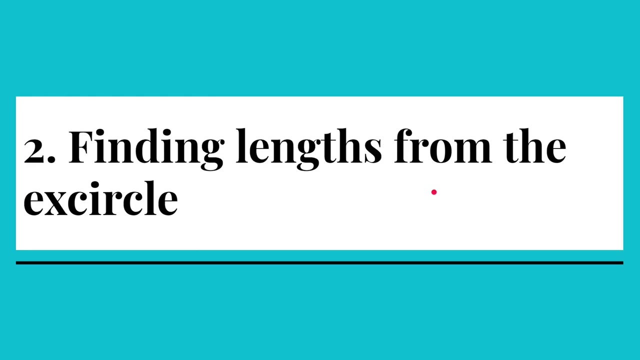 X is equal to S minus A, Y is equal to S minus B and Z is equal to S minus C. Hmm, these values look like something in Huron's formula. Hint, hint, hint. Part two: finding lengths from the X-circle. The X-circle is just like the N-circle. 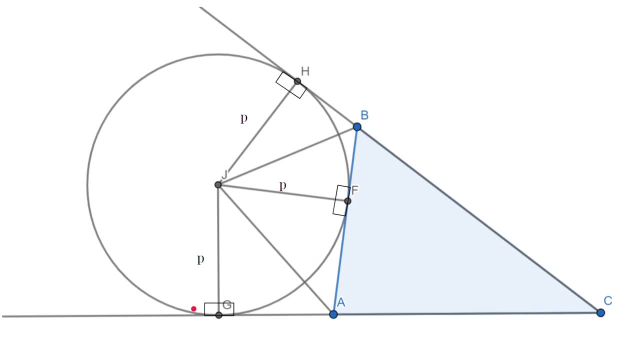 but it's outside of the triangle instead of inside it. Each triangle actually has three X-circles, one for each side, but we'll only look at one of them. for this proof, Let P be the X-radius, which is just the radius of the X-circle. We can notice that BF is equal to BH. 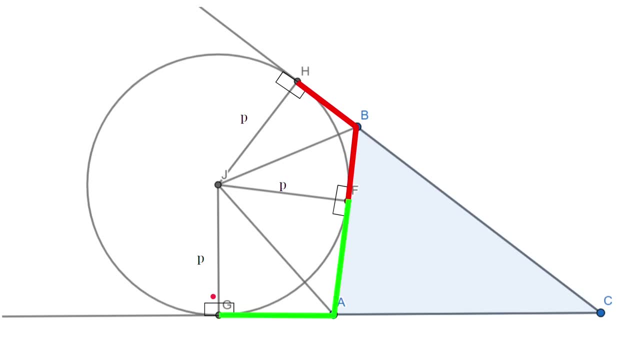 the red segments- and AF is equal to AG- the green segments- because of the ice cream cone theorem. So when we create these blue lines, we can fold them over to see that HC plus GC is equal to the perimeter of the triangle. And because of the ice cream cone theorem, 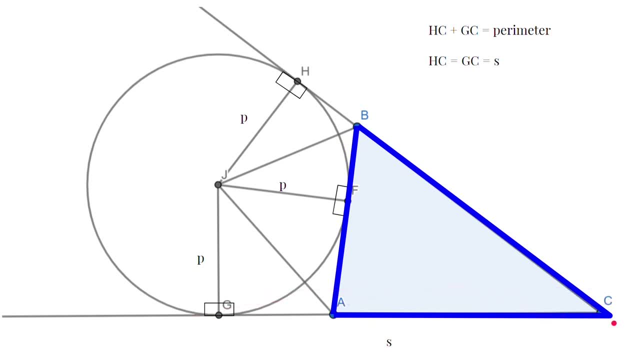 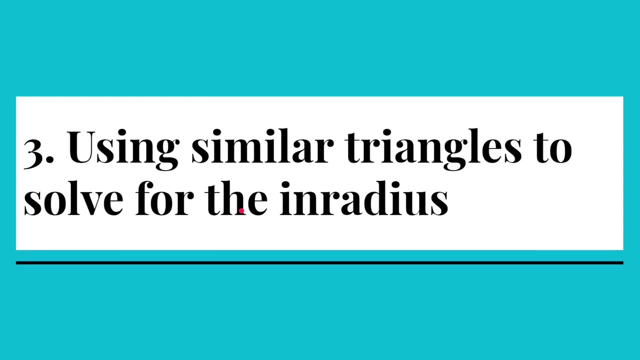 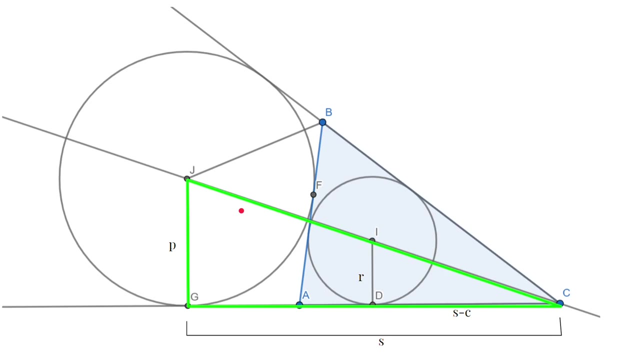 HC is actually equal to GC, So each of them is equal to exactly half of the perimeter, or S. Part three: using similar triangles to solve for the N-radius. Now, there are two pairs of similar triangles. The first is the red triangle and the green triangle, because they both have 90 degrees. 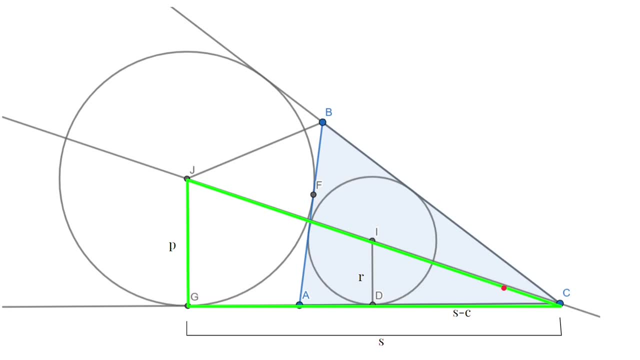 on the bottom And they both have this N-radius. Now, if we look at the red triangle and the green triangle, we can see that they both have the same angle. This means that the ratio of their side lengths is the same, because they're just scaled pictures of each other Using part two. we know. 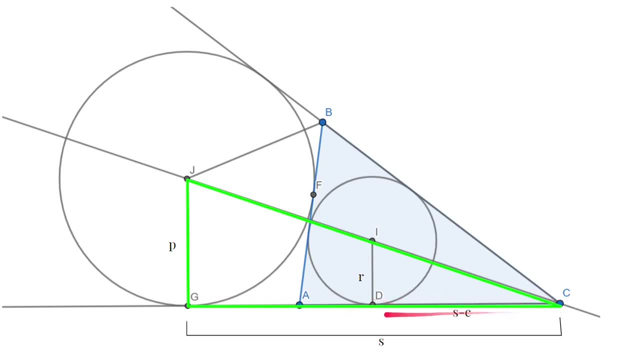 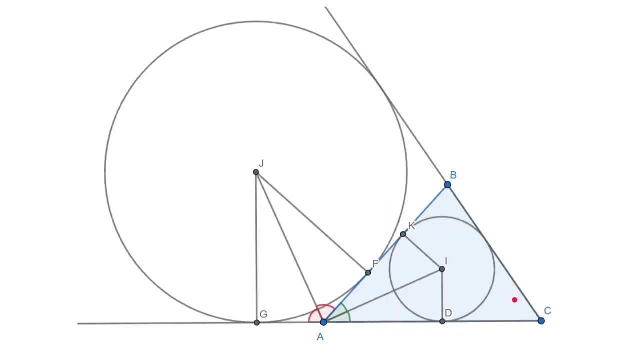 that GC is equal to S, And using part one, we know that this length is equal to S minus C. So plugging it all in, we get R over P is equal to S minus C over S. Now if we look at the red triangles, we'll need to look at the angles a little deeper. We'll first. 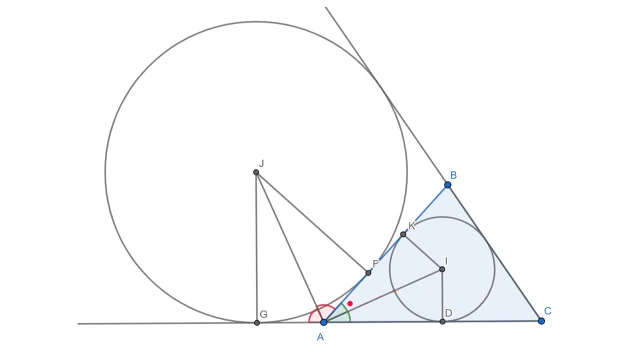 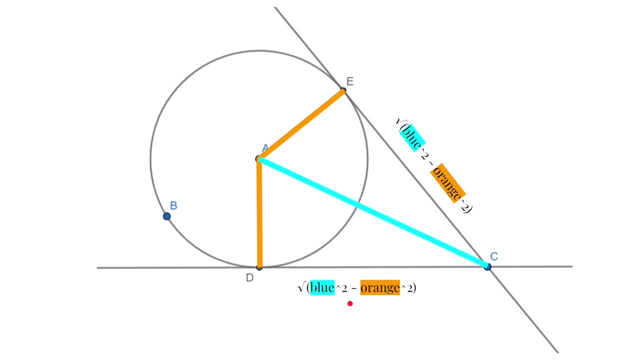 prove that the red angles are equal and the green angles are equal. Let's go back to our ice cream cone theorem picture. Since the two triangles have all the same side lengths, they are congruent and must also have all the same angles. So this is equal to this and this is equal to this. 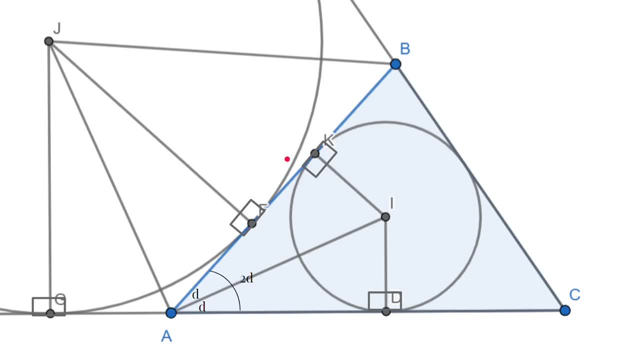 Let these two angles be D, Their sum is 2D, And since this line on the bottom is a 180 degrees, this is 180 minus 2D, And since these two angles are equal, each of them is 90. 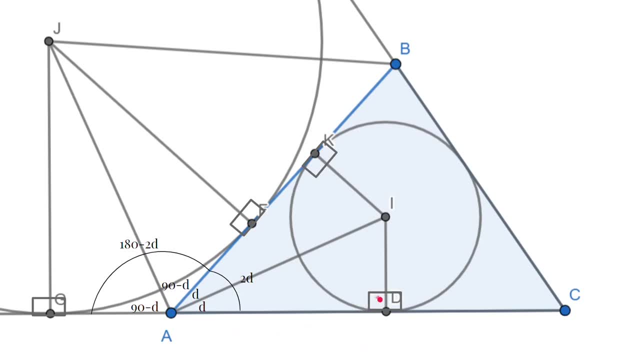 minus D. And now, since these are right angles and the sum of the angles in a triangle is 180 degrees, these are each 180 minus 90 minus D, which is 90 minus D. And by the same reasoning, 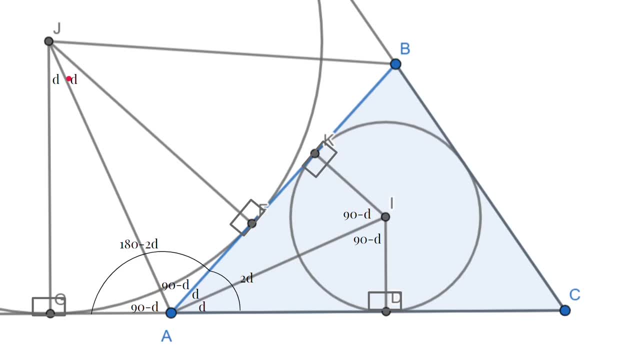 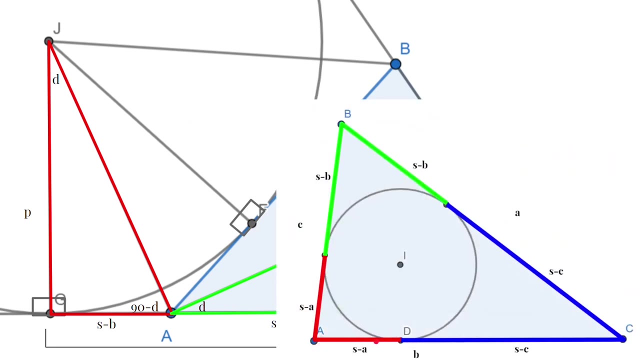 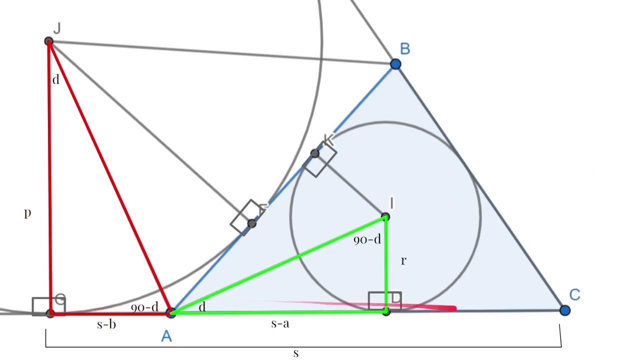 these are both D. We can see that the red triangle and the green triangle are similar because they have all the same angles. And now we can use part 1 to have: AD is equal to S minus A, And that comes in right here. And now we can use part 2, which shows that this long length GC is equal to. 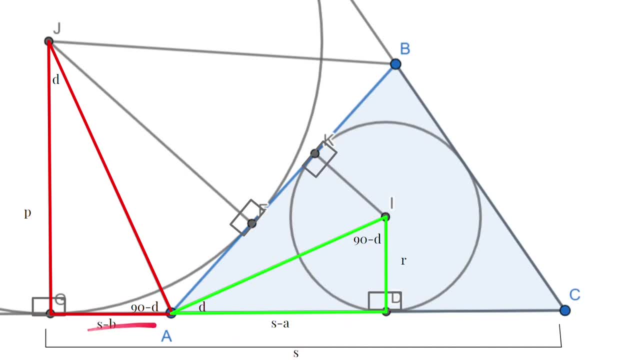 S, So this length is equal to AD. And now we can use part 2 to prove that the length of this long to s minus B, because this length is B. so since similar triangles have lengths of the same ratios, we have the s minus a over R is equal to P over s minus B, and we cross, multiply to get our P is s. 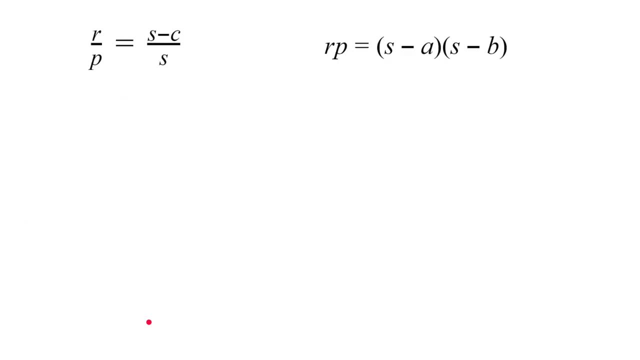 minus a times s minus B. okay, so now we have the quotient of R and P and the product of R and P. we're only looking for R right now, so we can multiply the two equations to get rid of P. and now we can just take the square root and get the. R is equal to the square root of s minus a times s.